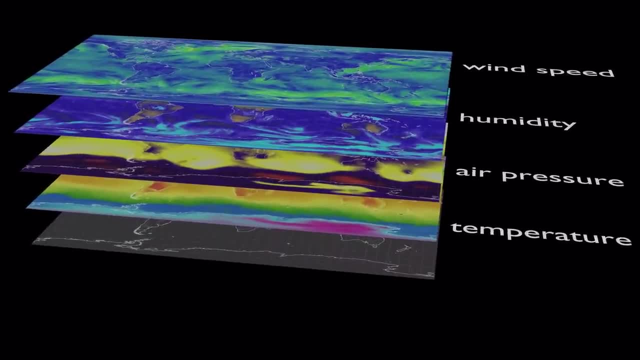 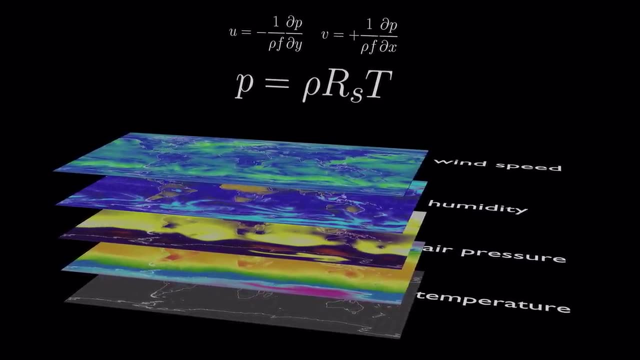 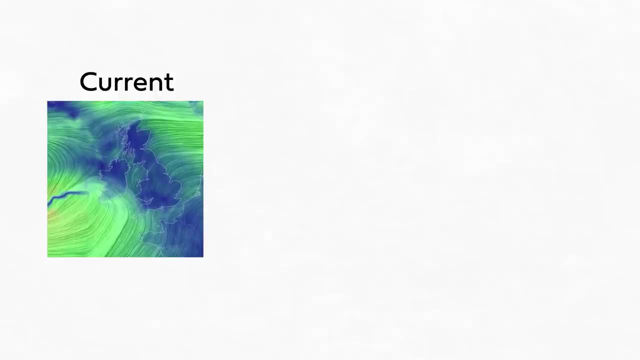 We can take the current state of the atmosphere, the values of pressure and temperature and so on, and, using these equations, predict what is going to happen at some time in the near future. The weather creates a future state of the atmosphere, maybe an hour into the future. 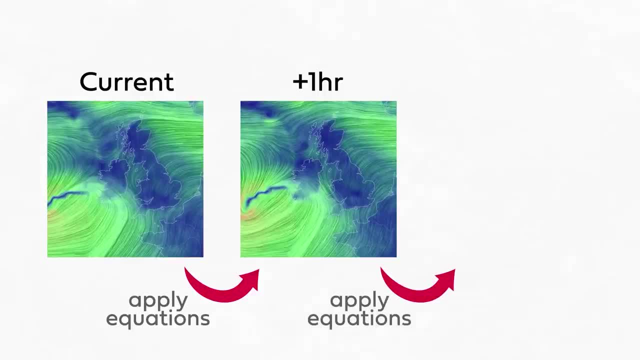 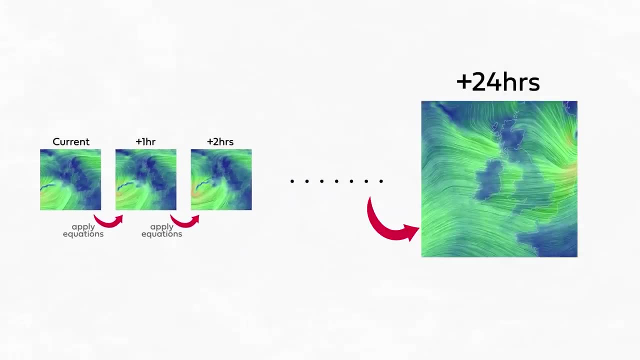 that you can then apply your atmospheric equations to again, to go another hour into the future, And you can do that again and again and eventually predict the weather 24 hours into the future and beyond, But to do that by hand producing an effective weather prediction. 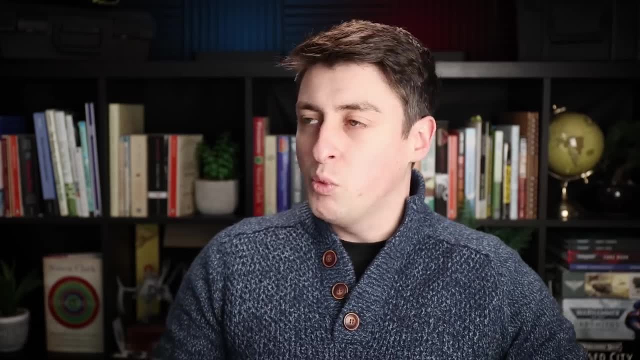 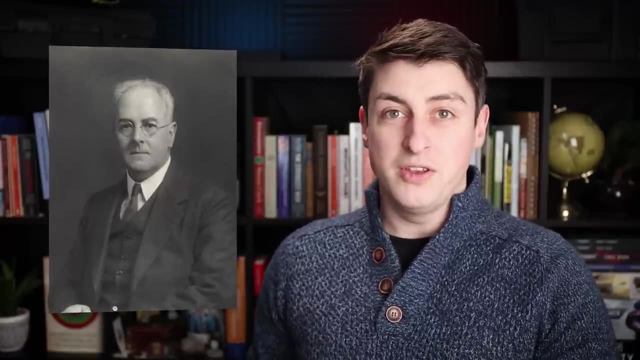 The weather creates a future state of the atmosphere. The weather creates an effective weather prediction. producing a weather forecast with pencil and paper would take months. Historical side note: someone called Louis Fry Richardson tried to do this in 1922.. If you want to learn more about that, you can read about it in my book, Firmament. 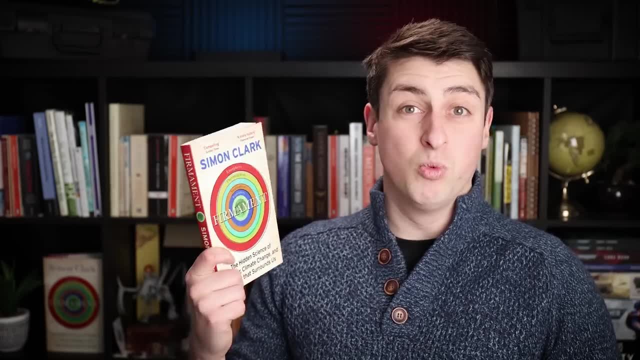 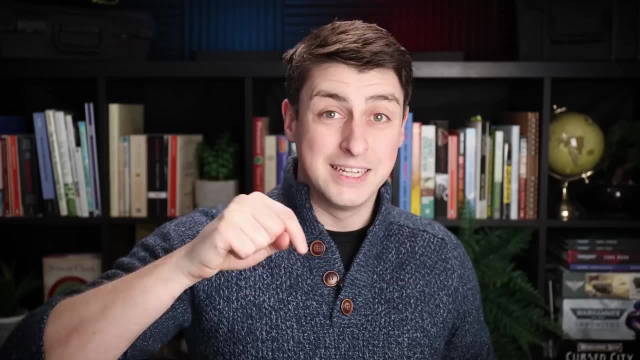 an introduction to and history of atmospheric science, named as a Waterstones book of the year and is now available as a paperback in the UK and Commonwealth and Europe, I think. I think it's all. floppy Link is down there in the description. Sorry, Americans, you get the paperback next year, I think. 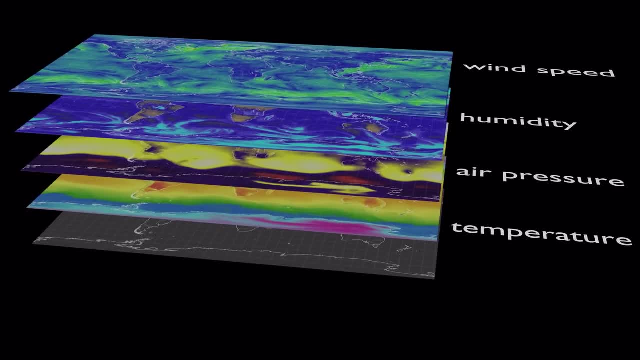 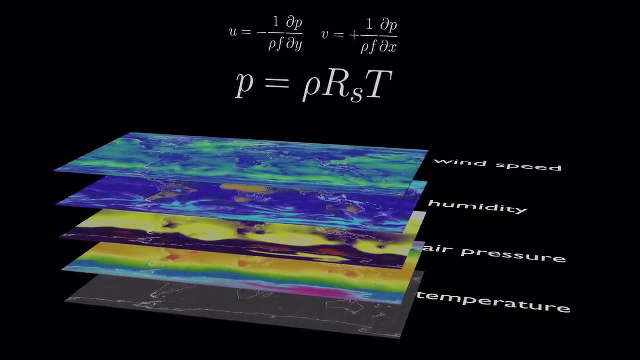 but the hardback is now available for you. Anyway, back to predicting the weather. To save us lots of time, we represent those equations describing the atmosphere in a way that a computer can understand and do for us. That means instead of describing the atmosphere over the UK, for example. 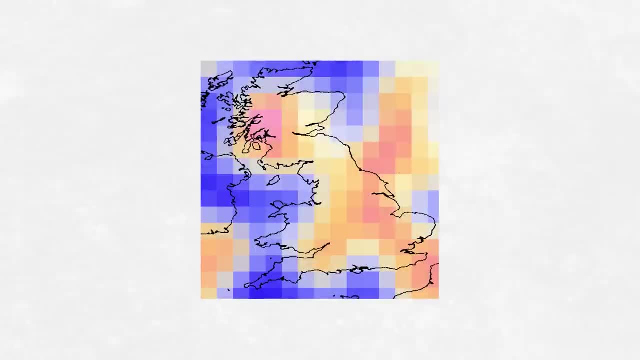 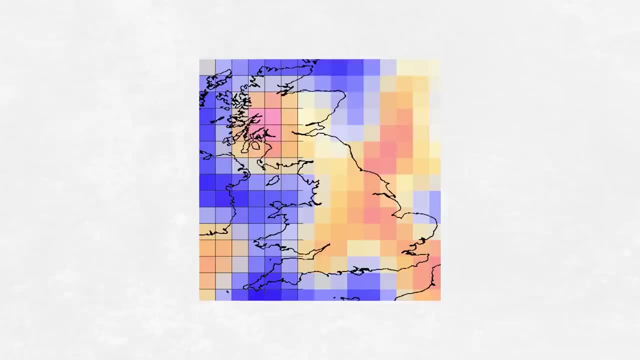 like this, smoothly varying. we describe it like this. We've broken it down into chunks or, to use the fancy term, discretized it. We measure the value of atmospheric variables on this grid and then apply the equations only at locations on this grid. 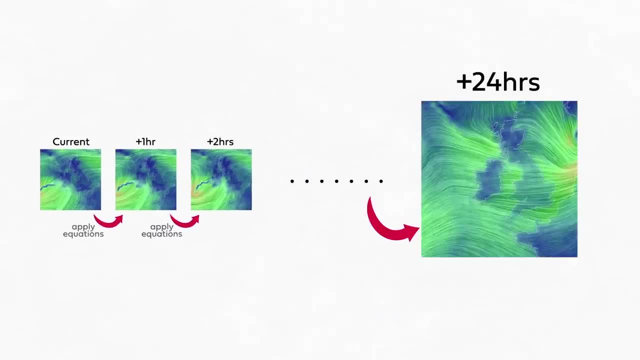 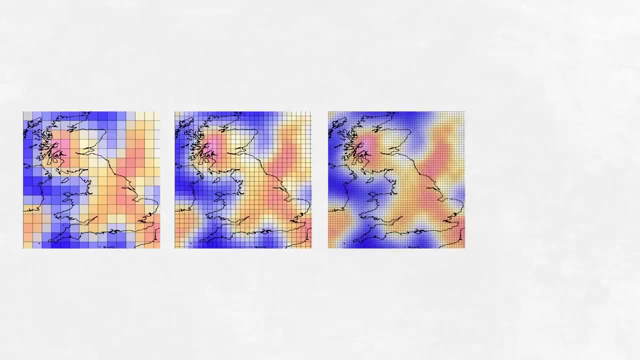 We can then iterate into the future, like I mentioned before. Of course, the more locations you do this for, the higher your resolution, the more accurate your approximation of the real atmosphere becomes In practical terms. you add as many points as your computer can tolerate without. 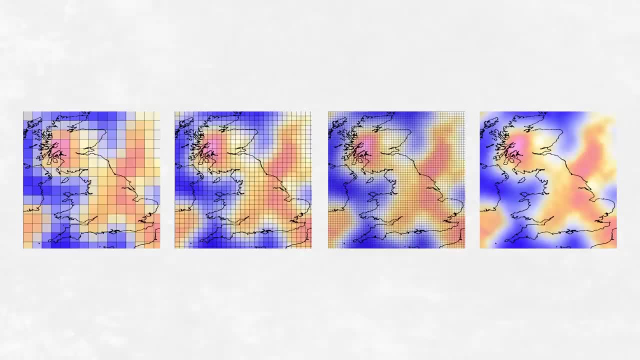 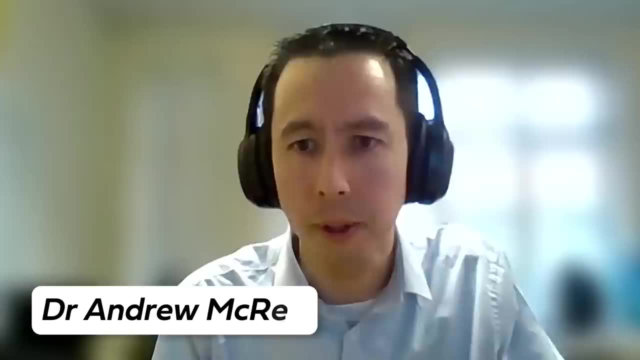 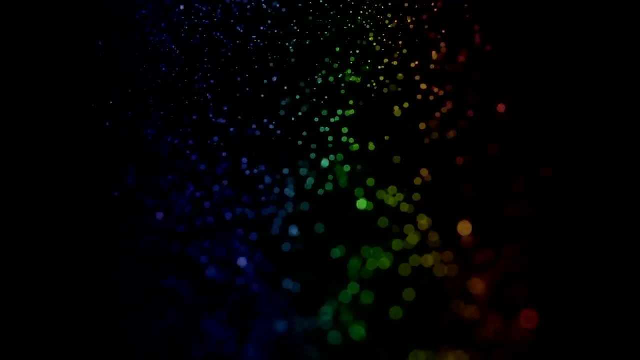 bursting into flames. doing the calculation, Most regional weather prediction models have points that are a few kilometers apart. But why is that a problem for rainfall? specifically Physical processes that lead to rainfall. they happen well below the resolution of the typical weather forecast computer models that we have. 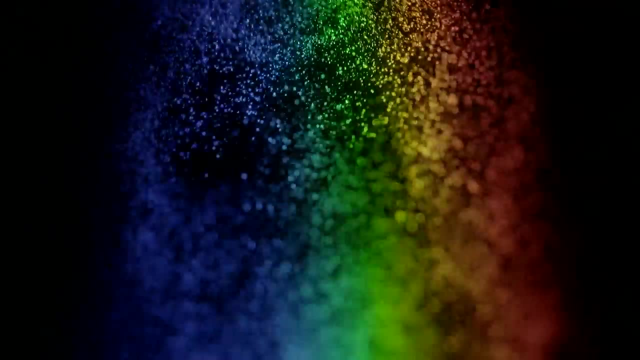 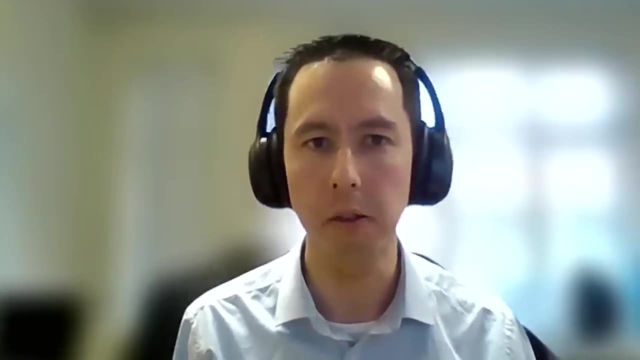 These processes are things like water vapor condensing around little impurities within clouds, also convective updrafts and downdrafts that lead to intense rainfall. All of these are happening well below the resolution of the models, which is typically one kilometer for local models and maybe 10 kilometers for global models. 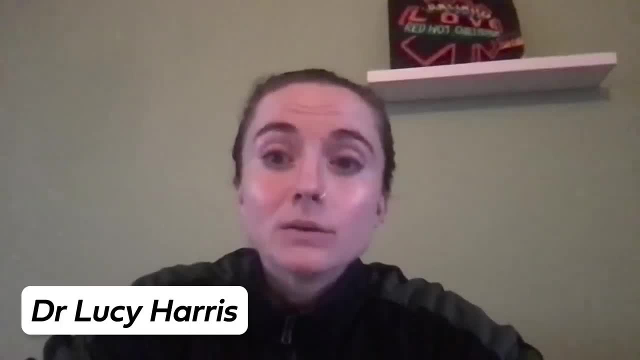 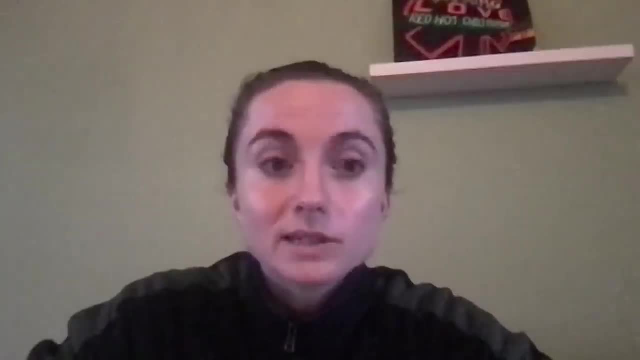 The end user really needs to know on quite a local scale whether or not it's going to rain, but also, ideally, how much it's going to rain, And precipitation varies quite sharply over small scales, So you can measure that in terms of in-your-house estimation. 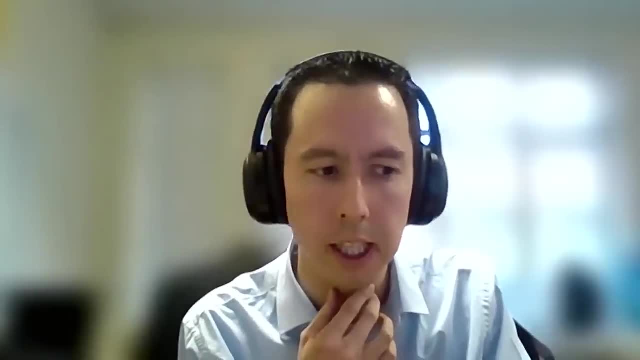 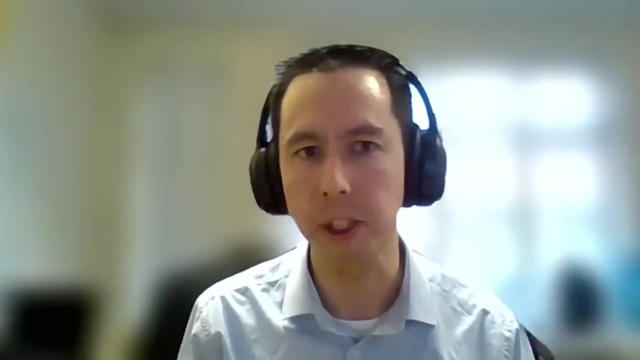 And, as a result, these processes that lead to rainfall. they are what we call parameterised, And that really means that they're very crudely approximated within the models And therefore the resulting predicted rainfall can be really quite inaccurate. This is Dr Andrew McRae, and he's joined by Dr Lucy Harris. 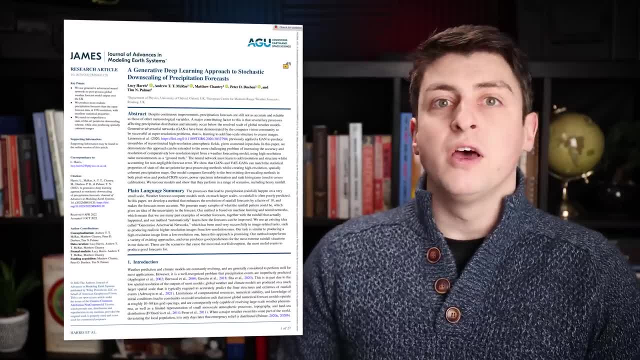 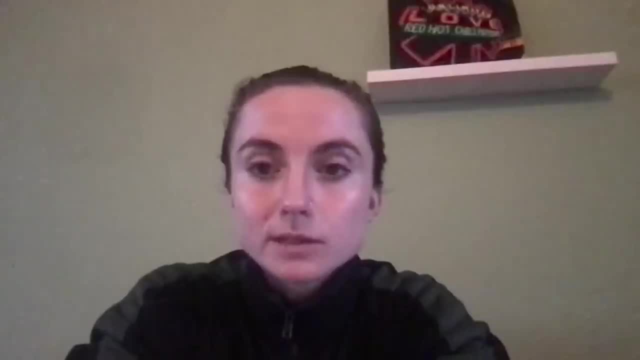 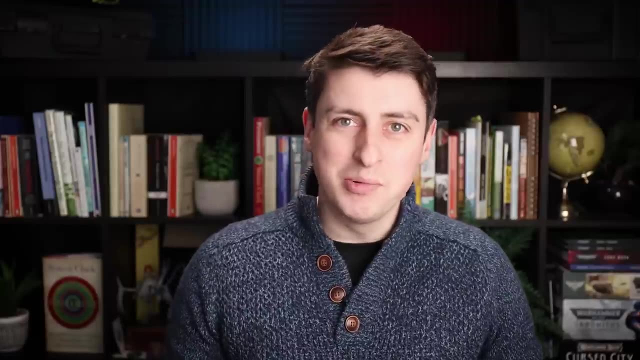 two of the authors of this paper that was published late last year that improves the forecasting of rainfall over the UK using machine learning techniques. So we use a machine learning technique called a generative adversarial network to achieve our downscaling. This may sound complicated, but the idea is actually very similar to a tool that you may have used. 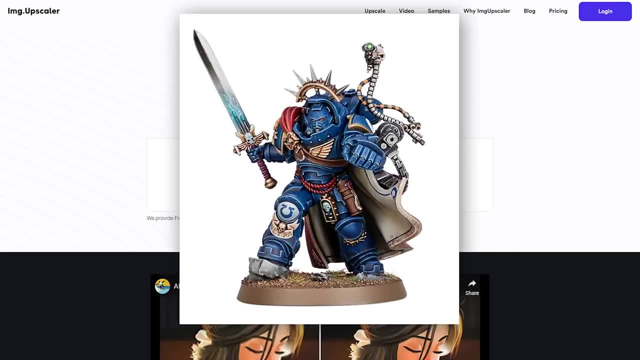 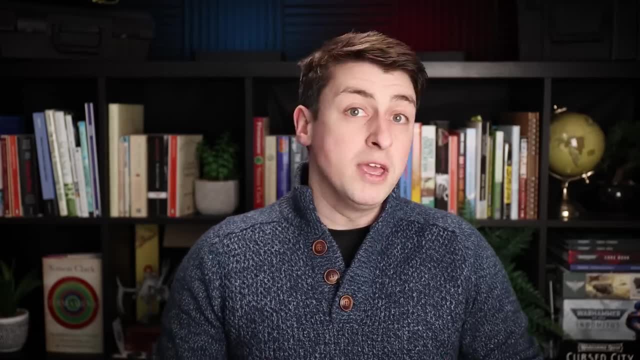 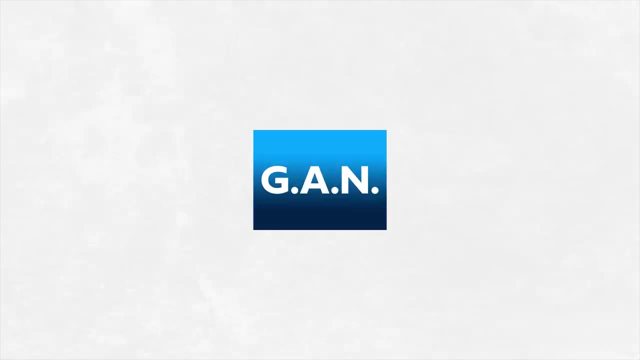 Websites like imageupscaler allow you to input low resolution images and, through machine learning techniques, receive higher resolution images. These tools are upsampling or improving the resolution of the image. Similarly, the generative adversarial network, or GAN, from the paper takes in the low resolution output from a global weather prediction model over the UK. 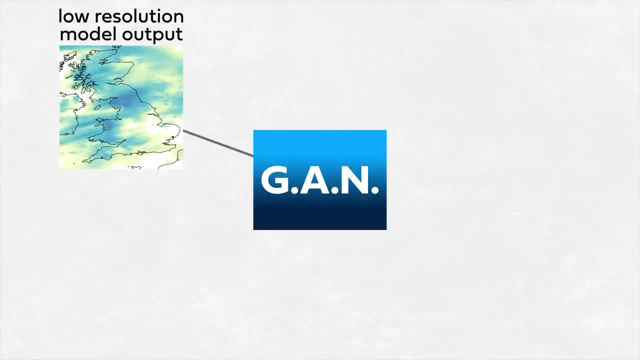 information such as pressure, temperature and humidity on the low resolution grid, but also some extra information like a high resolution map of the height of the landscape of the UK. and then does its fancy maths magic- It's really just linear regression- And outputs a higher resolution weather forecast for the UK. 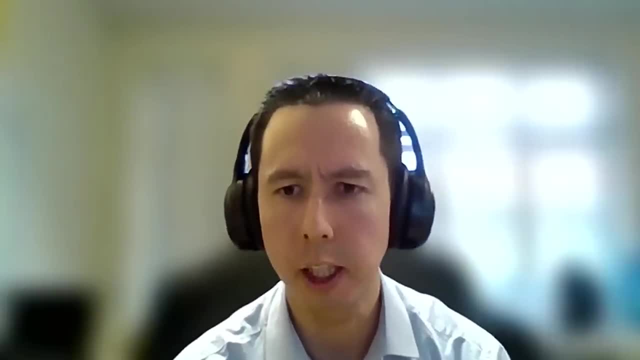 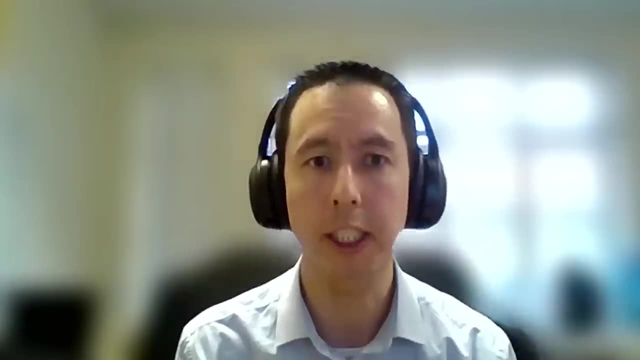 So it's very similar to the idea of things like image upsampling that's used in computer graphics. One thing that's quite different in the work that we've done is that our model takes into account, basically, that the weather forecast can be wrong. 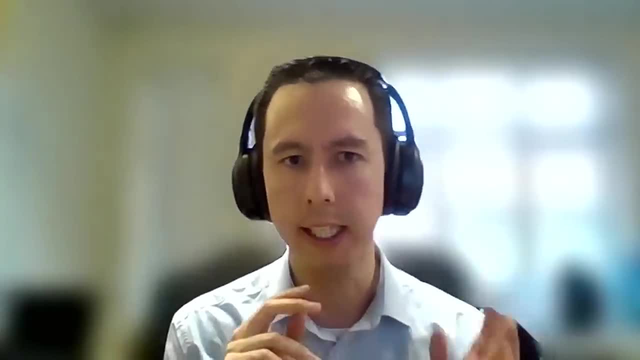 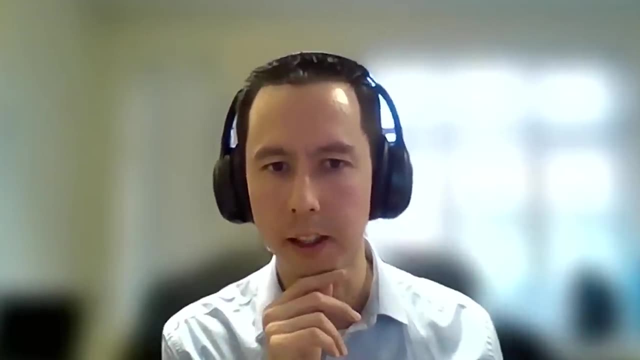 So our model: we take in a single weather forecast, we train it against a separate data set, a radar based data set of what actually happened and of course there's going to be differences, So it's not just that one of them is higher resolution than the other. 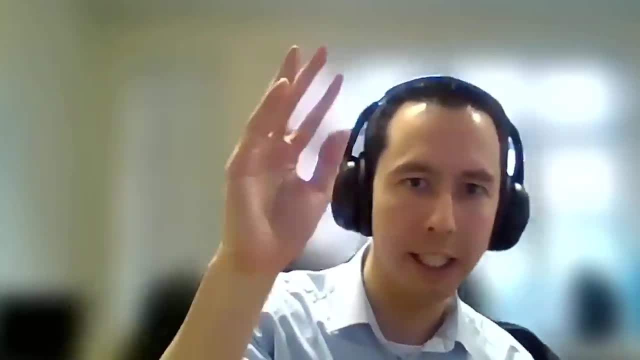 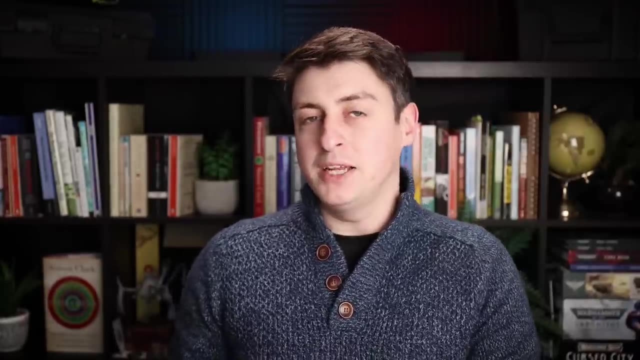 but it's also that the weather forecast said the rain would be here, and actually it was here. But that's not all. There's a fundamental difference between an image upscaler and this paper, and it's to do with the nature of the atmosphere. The atmosphere has a very sensitive dependence to initial conditions, and so if your model has taken the cloud to slightly the wrong place, then even without all of this issue with the parameterizations, the rainfall is still going to fall in the wrong place. Any uncertainty in how you initialize a forecast? such as not being exactly sure what the temperatures are at all your grid locations- something that, by the way, is inevitable- and the error in your forecast will grow exponentially over time. That's chaos theory. One way to tackle that is to use stochastic models. 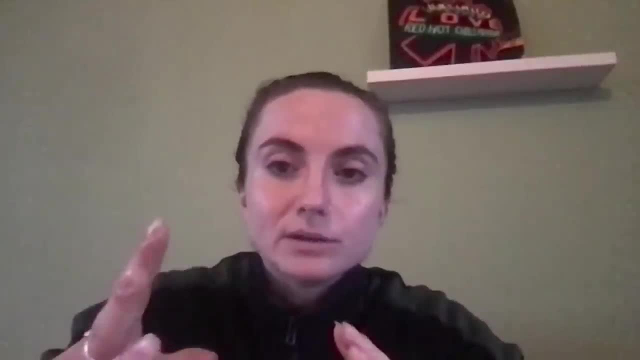 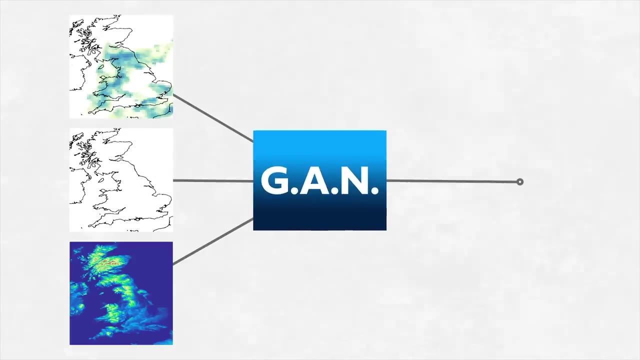 where you have a slight amount of noise added to your input- sort of just random noise- and you see how much of an effect that has on the output. So if we're slightly wrong about the initial conditions, do we come to the same conclusion? 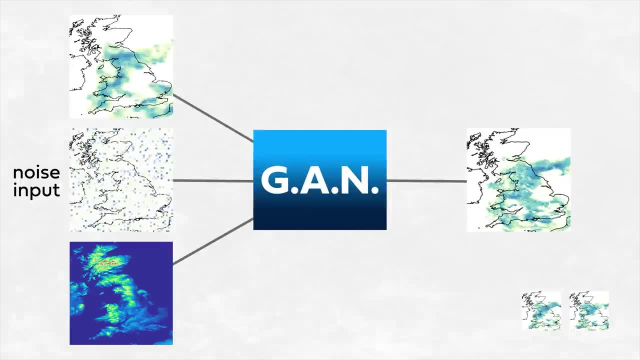 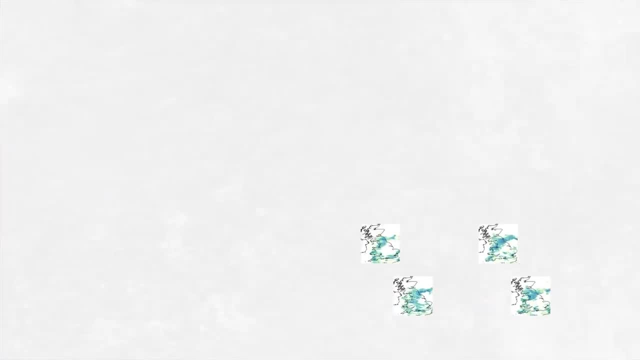 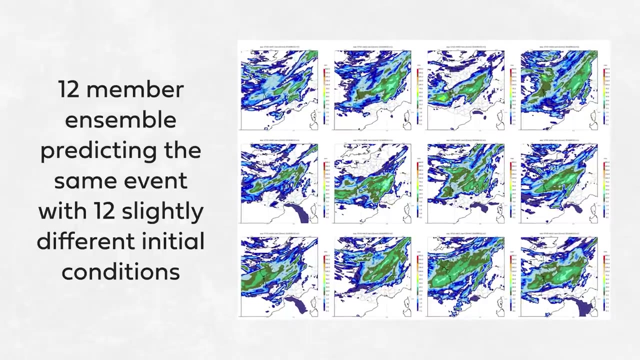 or are we wildly diverging away? So the stochastic model tries to give a probabilistic representation of the set of conditions, of possible outputs, given a slight uncertainty around the initial conditions. And this is how weather forecasting is done. You don't just get one forecast out of your model. 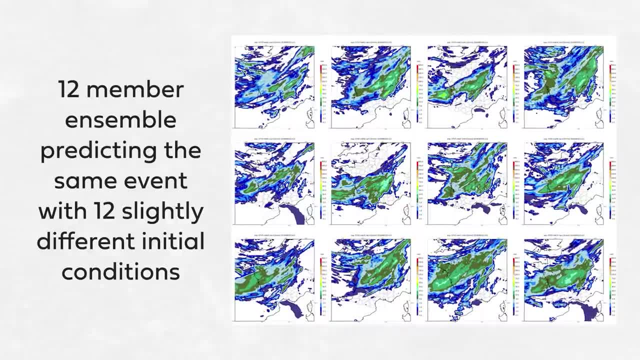 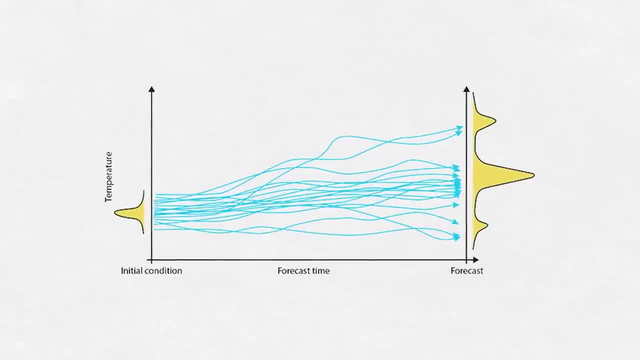 you generate an ensemble of outcomes, given slightly different inputs, which can tell you the most likely forecast, but also tell you how certain you can be about that forecast. The tool that Lucy and Andrew and others have put together is an extension of that idea. 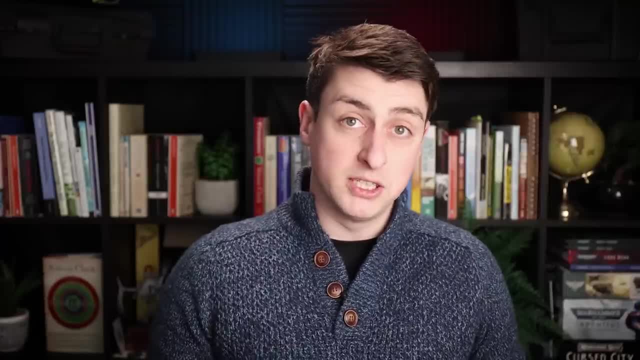 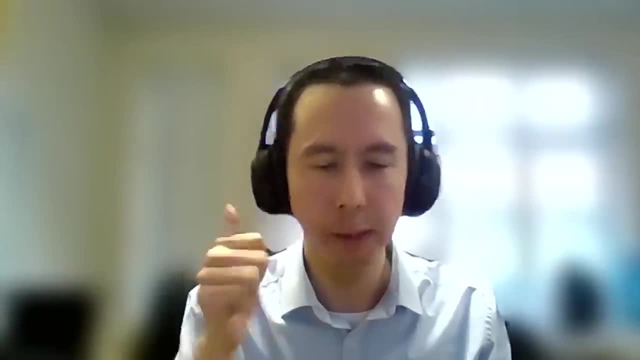 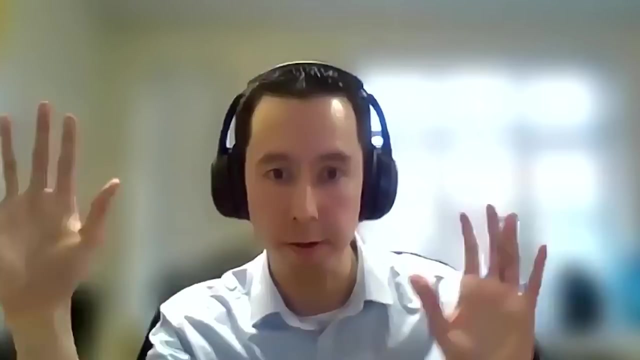 married with machine learning techniques and provides post-processing to rainfall forecasts. specifically, I'd say that our model does three main things really. So number one: it can correct biases. If you produced a large number of ensemble forecasts and took the average, then that would be different to the input. 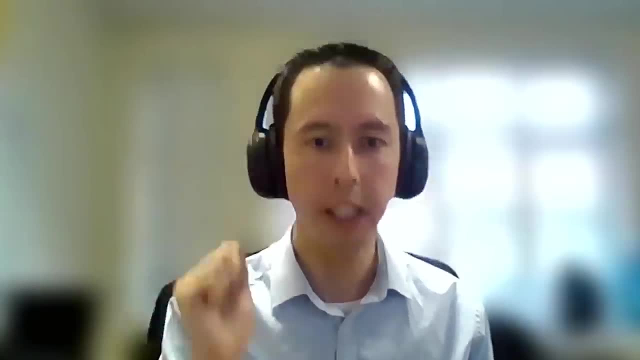 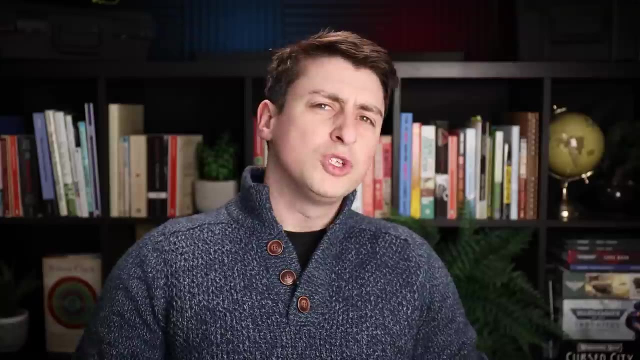 So that's correcting the bias. Number two, it adds variability. And number three, it increases the resolution. So somehow our generative, adversarial network approach is doing all three of those things at once. So, considering how effective this tool is- and the paper is clear- it is effective. 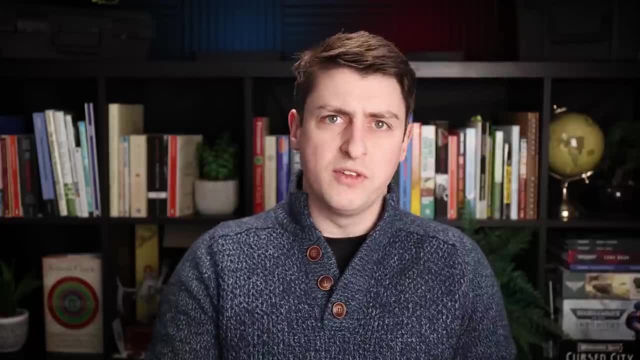 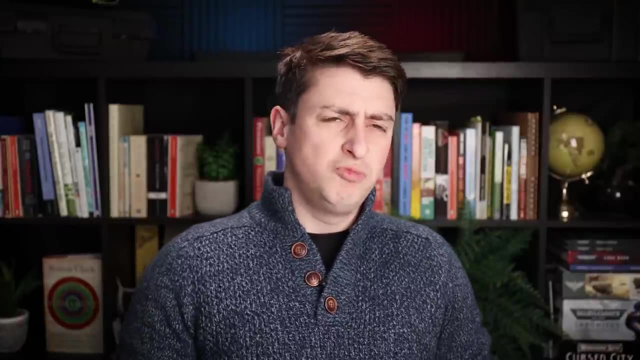 you may well ask: why don't we use more machine learning in weather and climate prediction? In fact, why even bother creating really complicated weather forecasting models and just let machine learning do the whole thing? Well, there have been some very exciting papers that have come out. 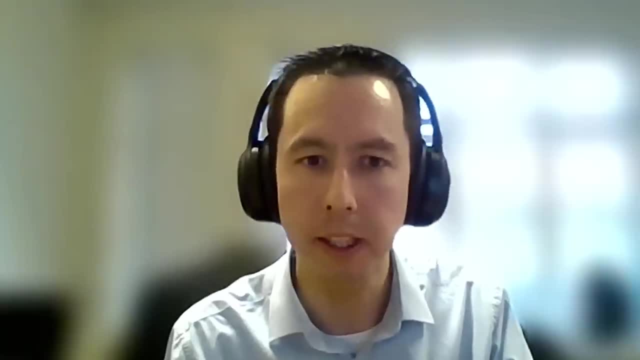 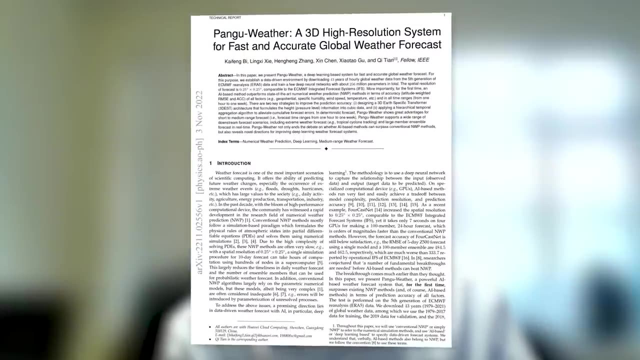 in the past couple of years, Literally within the past few months- there's been a couple more huge papers that have dropped: One by Huawei with a model called Pangu Weather, And just before Christmas there was one by DeepMind. I've forgotten what they call their model, but 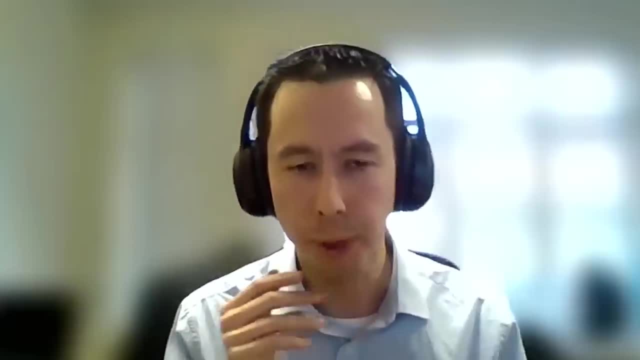 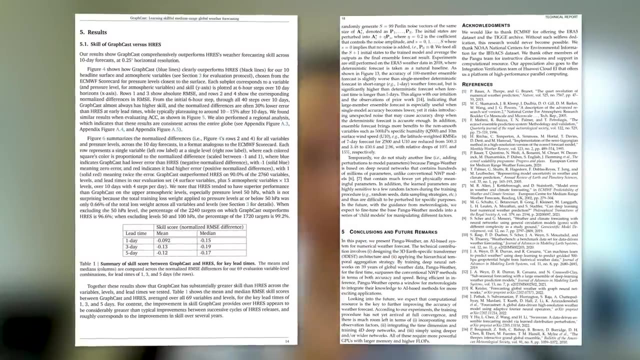 It's called GraphCast the paper by DeepMind. These are purely machine learning based models, And these last two papers particularly so: Pangu Weather by Huawei and the DeepMind paper. they've shown that their machine learning model is basically on a par with the best existing weather models. 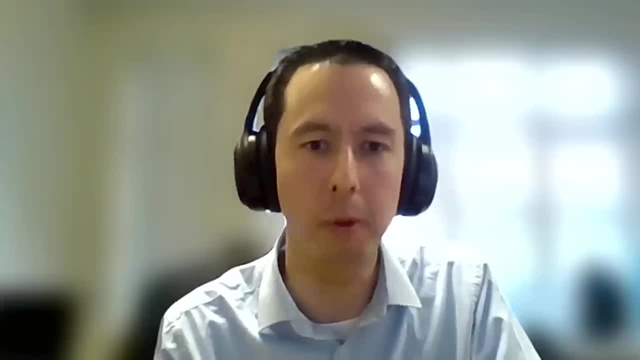 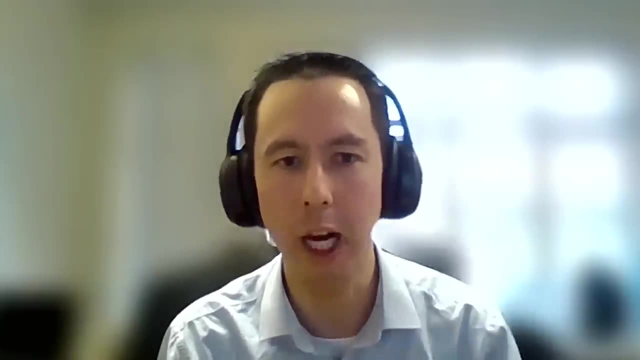 maybe better. I think the rate of progress is just so vast that I would not be surprised anymore if, a few years from now, the machine learning model, the latest models, outperform the existing models by far, For now at least, post processing using machine learning techniques. 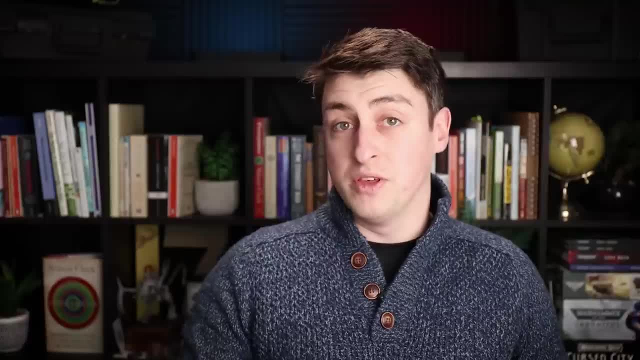 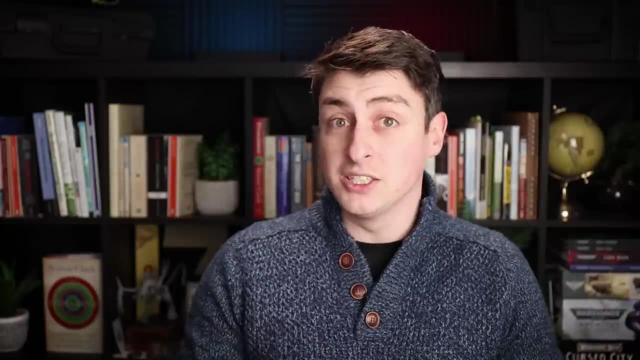 such as described by this paper, is a valuable tool in weather prediction and, going forwards, may provide a crucial tool in predicting extreme rainfall events and thus disaster relief, as well as, you know, reminding you to pack a raincoat Now, now, now, now, now, now. 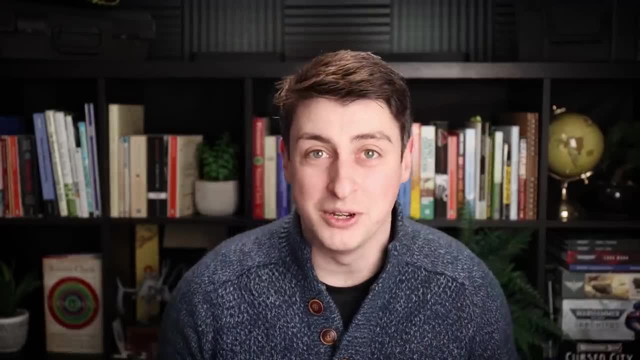 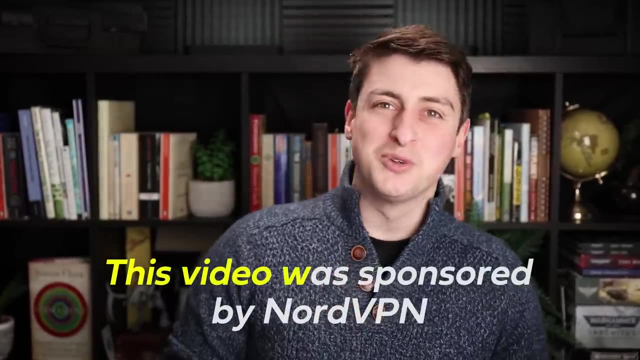 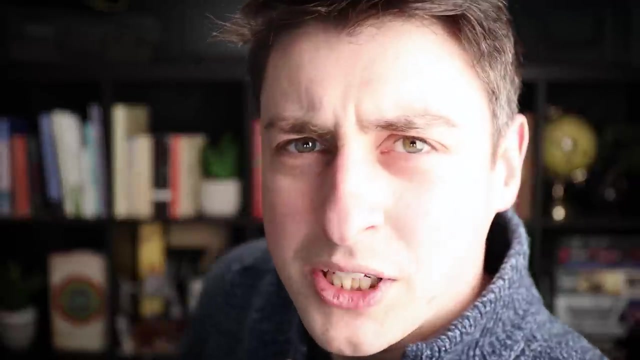 now. I am delighted to announce that I have reached a milestone in my YouTube career. join in with this one. bring up the karaoke lyrics, because this video was sponsored by nordvpn. we did it, everyone. we did it. give me a high five. but what is a nordvpn? i hear you ask. a vpn is a. 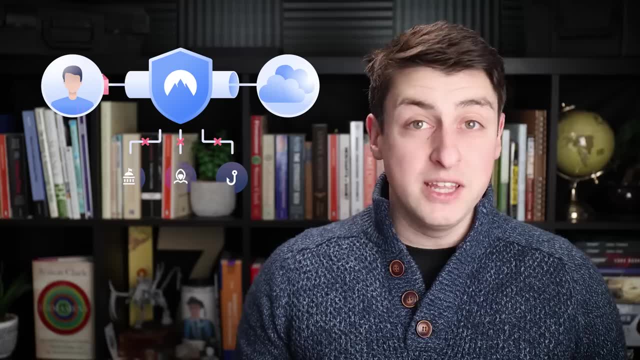 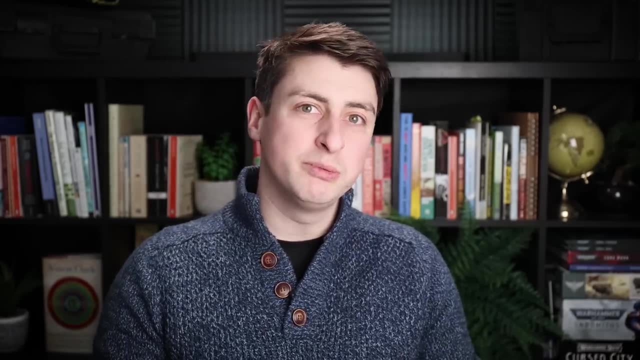 way of obscuring your ip address, making it appear as if you're browsing the internet from another location that you can choose. that has privacy benefits, but it also allows you to access location-specific services. for example, in the uk and want to watch tv that's only available on? american streaming services. get nordvpn set your location to be in america. want to save money up to 85 on renting a car? get nordvpn set your location to be in the cheapest country for the service. i've personally used nordvpn for several years now, mostly to access location specific stuff. 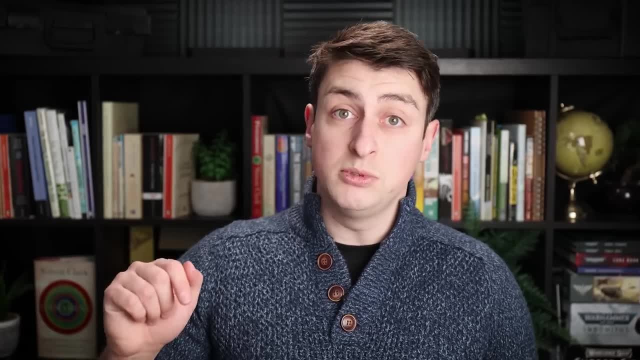 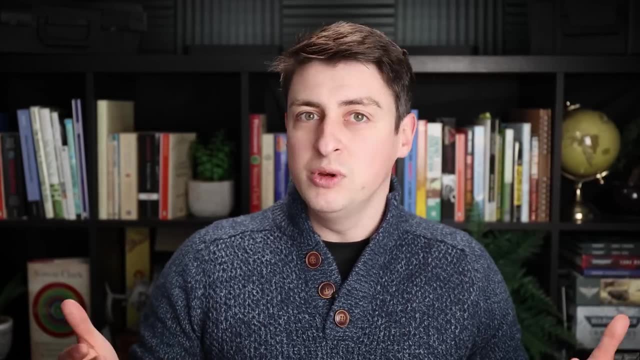 and i can categorically say that several videos on this youtube channel would not exist if i didn't have access to nordvpn's features. it's just a really genuinely useful tool, but as well as being useful, you can also get NordVPN for free, with a free raffle, from the link on the description of this video. 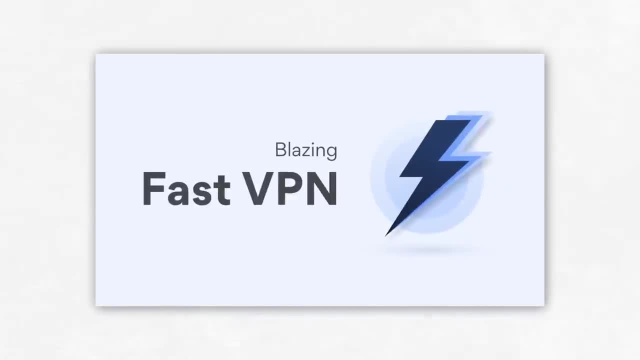 and you can also get NordVPN for free, with a free raffle, from the link on the description of this video. Useful, it's easy to use the fastest VPN out there and you can cover 6 devices on the same plan, And all that costs just a few quid a month. 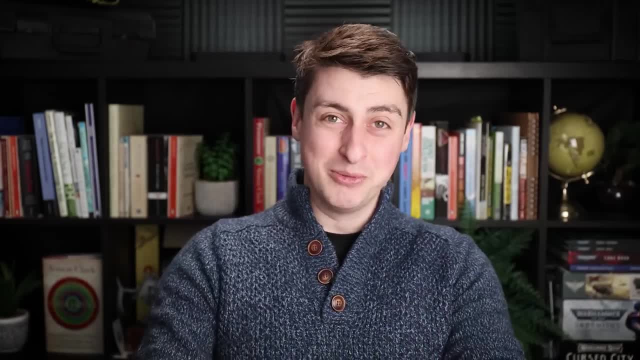 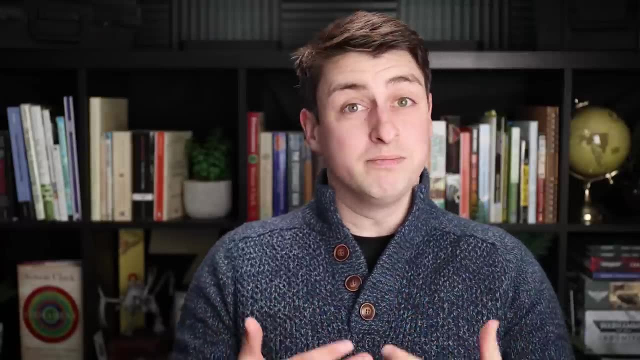 This isn't an exaggeration, this isn't a bit. I am genuinely delighted to be working with NordVPN on this sponsorship. it's like another gemstone in my YouTuber infinity gauntlet. I think it's a great service. I use it. I think you'll like it too.